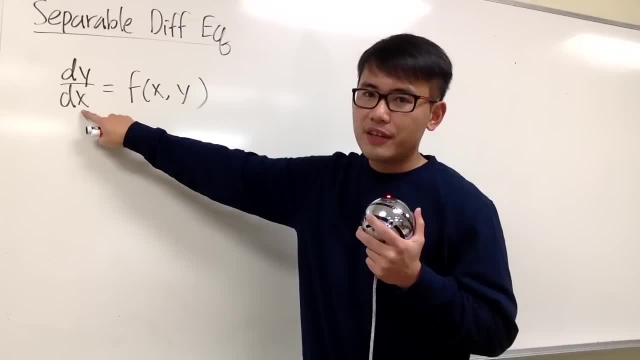 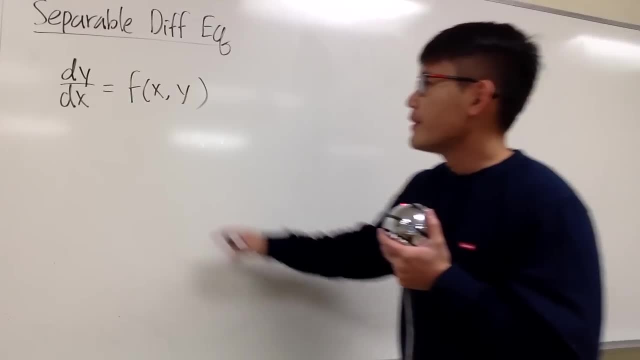 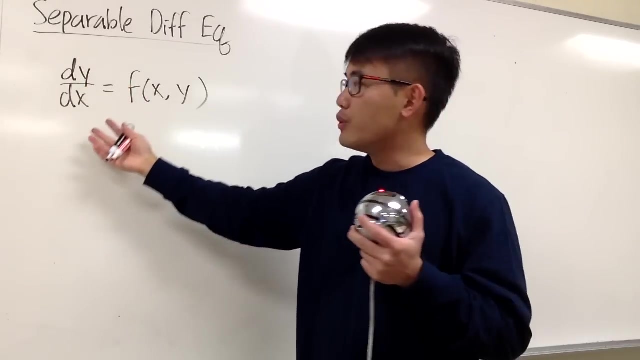 right, And you see, this is just the first derivative. Therefore this is also considered to be the first order differential equation. Sometimes this can be written as y prime. In that case, just write it down as dy over dx. Maybe we are using t for the independent variable. 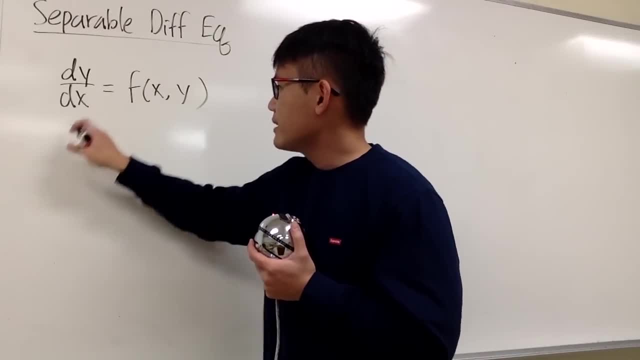 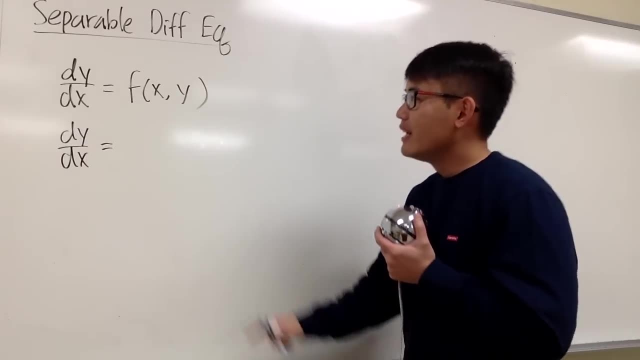 then dy dt, then things like that. All right, let me write this down again: dy dx. Our goal is to focus on the right-hand side first. This right here is a function in terms of both x and y together. Our first job is to separate. 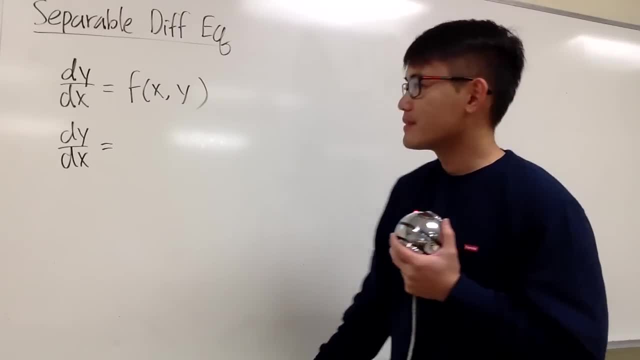 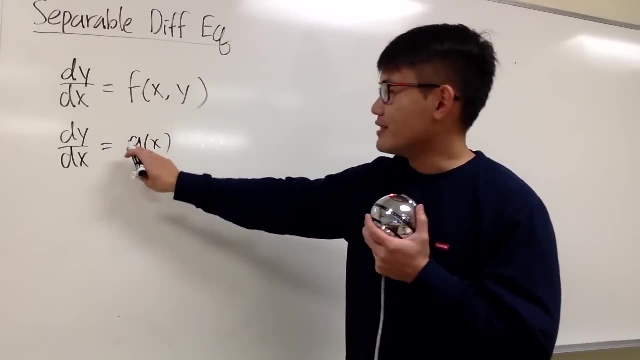 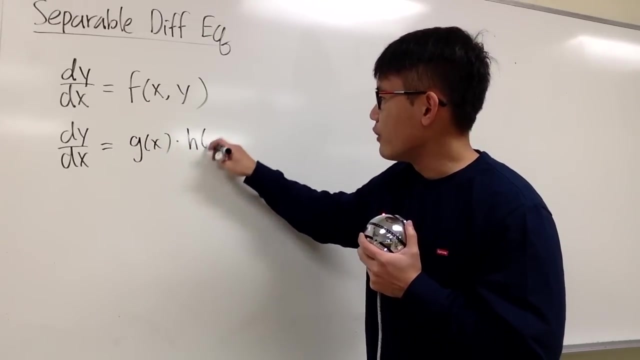 the x and the y by factoring. Look at the right-hand side. I want to factor it as a function and I will just write it down as g of x. It's an expression in terms of just x. The second part is going to be multiplying with h of y, a function in terms of just y. 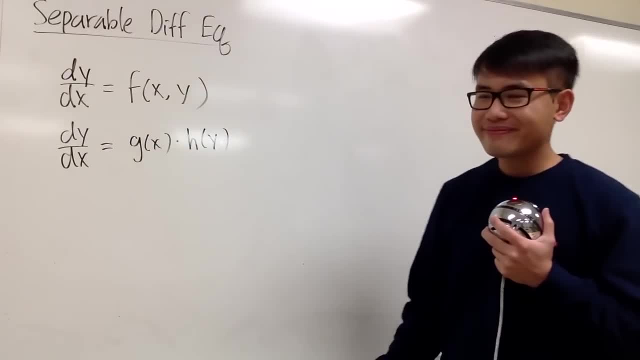 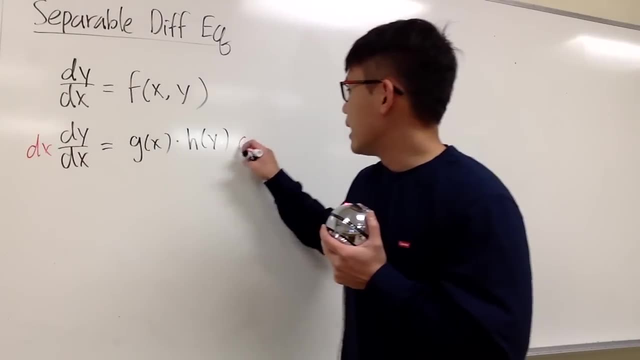 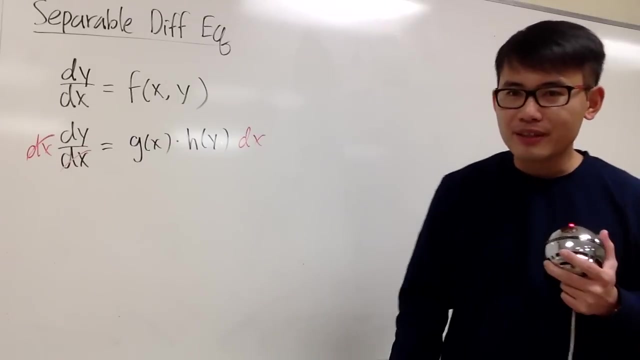 And this is what we mean by separating the variable. Next, I'd suggest you guys to do it this way: Let's multiply dx on both sides. Whenever we're trying to solve a differential equation, the differential should not be in the denominator. So let's take care of that first, and then we will have dy equals to. 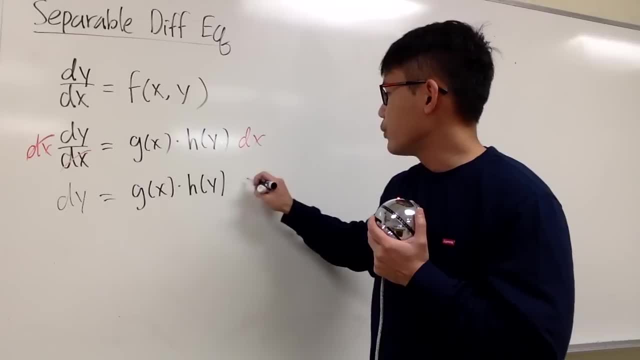 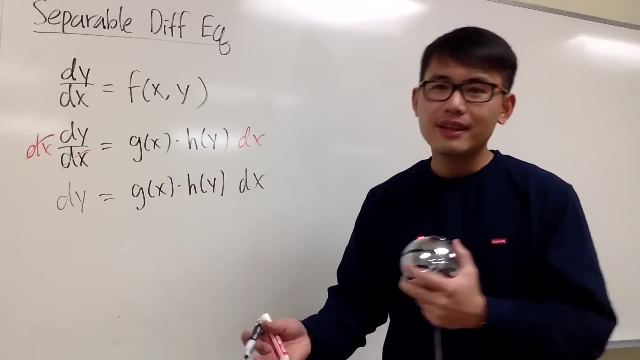 g of x times h of y, and then we have the dx right here. and then what you want to do is you want to have all the y's together on one side and all the x to get on one side. you see, we have h of y, right. 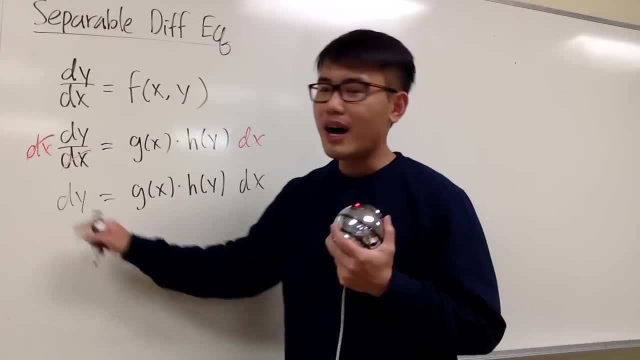 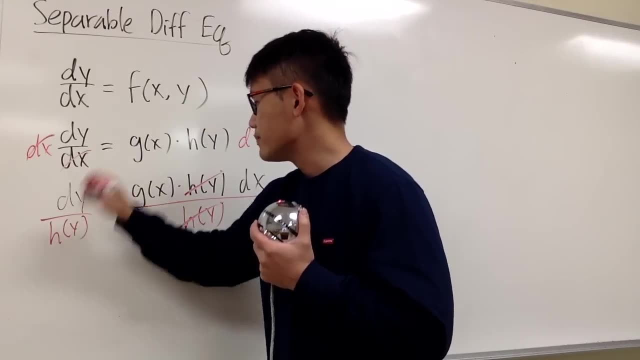 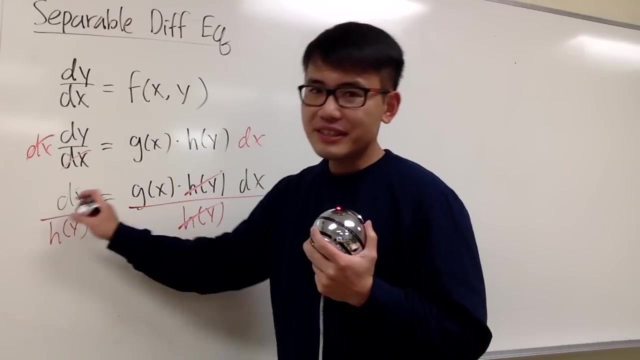 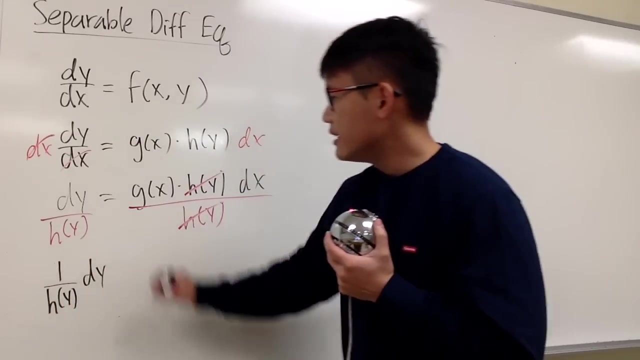 here. that should be together with dy. so let's divide both side by h of y, so they cancel. now divide this by h of y as well, and the g of x is together with dx, so that's great. on the left hand side, let me write this down as 1 over h of y, and then let's put a dy on the side, and this is equal. 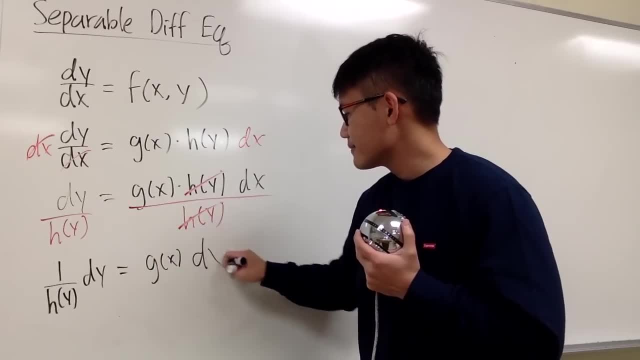 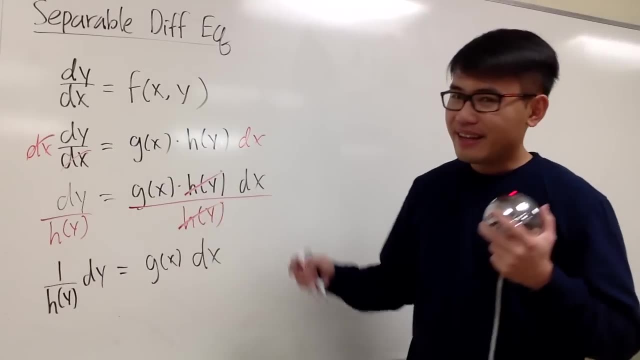 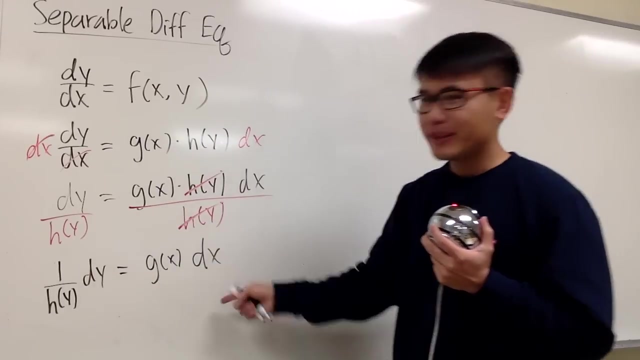 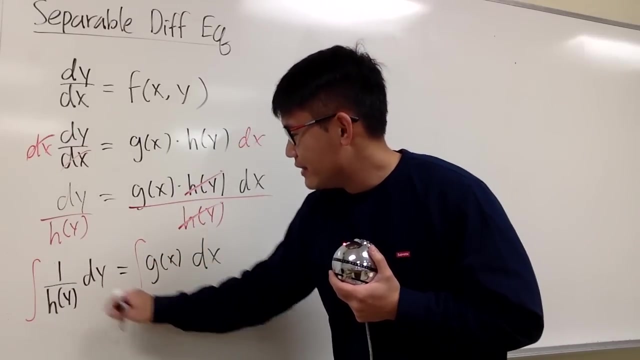 to g of x, dx, and you see, this is what we mean by all the y's together and all the x together, and congratulations to so you, this kind of differential equation. all we have to do is integrate this and integrate that. so we just have to do the integrals twice. okay, and hopefully this is not bad to integrate. likewise, this is not. 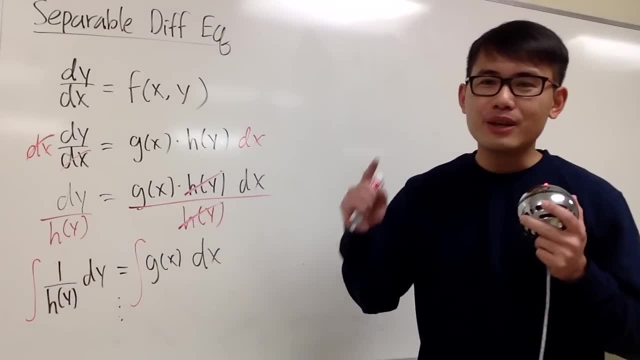 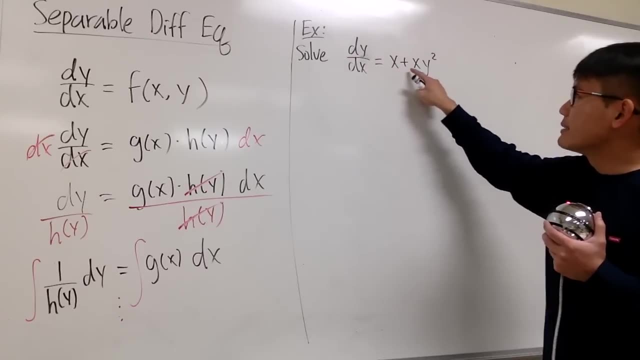 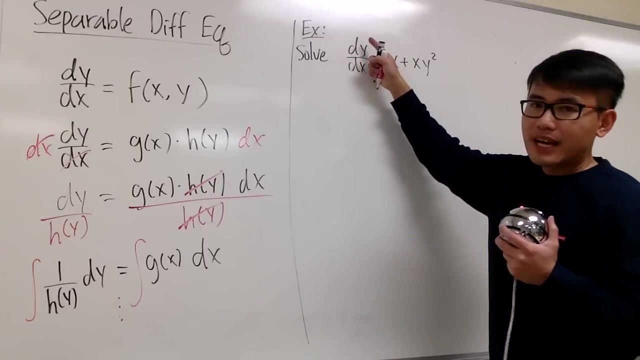 bad to integrate as well. and now let's take a look of an example. let's take a look at how we can solve this differential equation we have: dy dx is equal to x plus x times y square. as i mentioned earlier, the strategy is have the dy dx on one side, which we do right. so now let's focus on the. 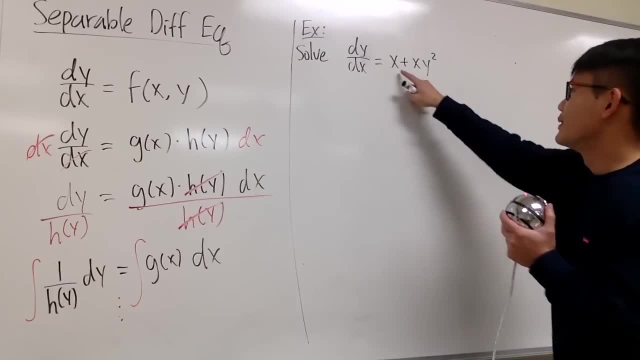 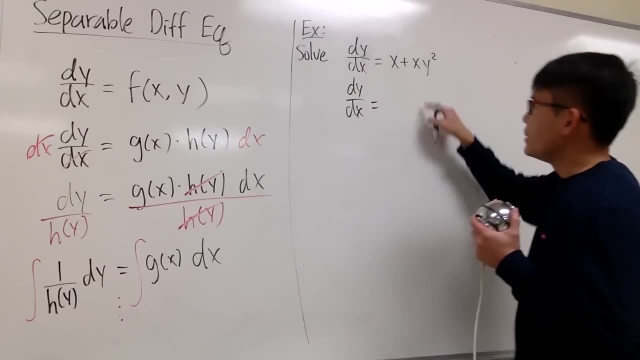 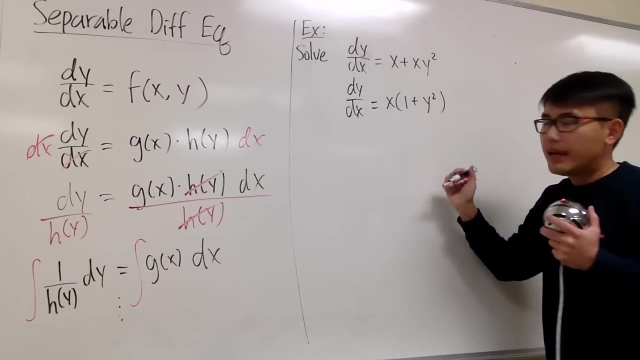 right hand side. can we factor things out? yes, we can factor out the x, because both terms have the x, right. so let me write this down again: dy dx, this is going to be. let's factor the x. so we have x in the front and we have 1 plus y squared like this. and now i want to show you guys all the. 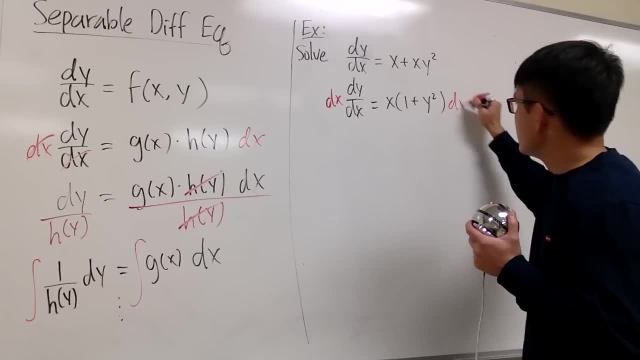 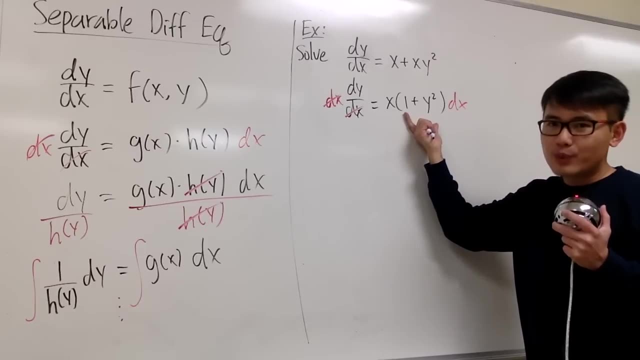 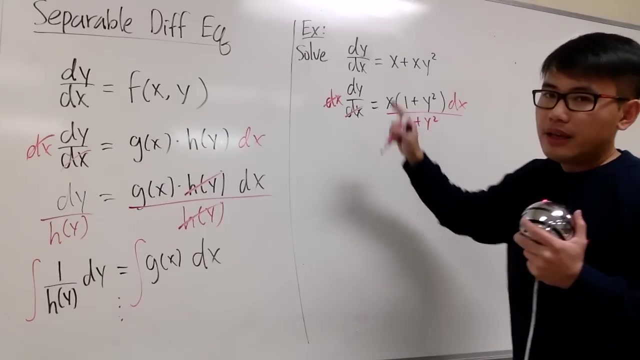 steps. let's multiply dx on both sides. this way, dx will cancel and we'll have this right and we have to divide the 1 plus y squared on both sides so we can bring this to the other side. so let's do that: divide this by 1 plus y, squared, and right. 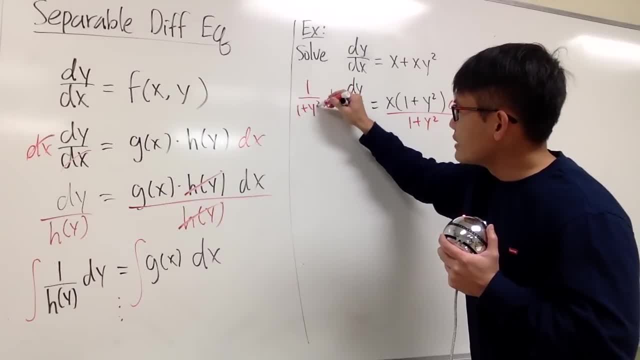 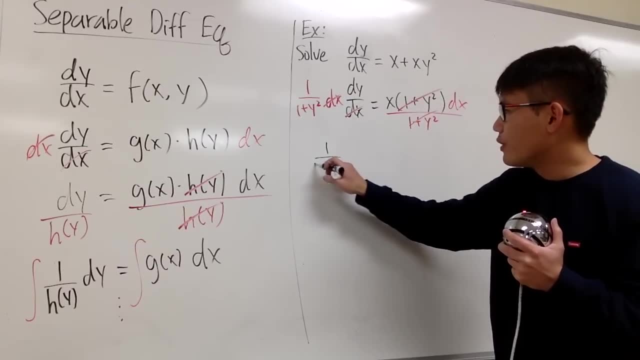 here. let me write it down as 1 over 1 plus y squared, and then, you see, this will cancel. on the left hand side now we'll just have 1 over 1 plus y squared and let's put a dy on the side and then 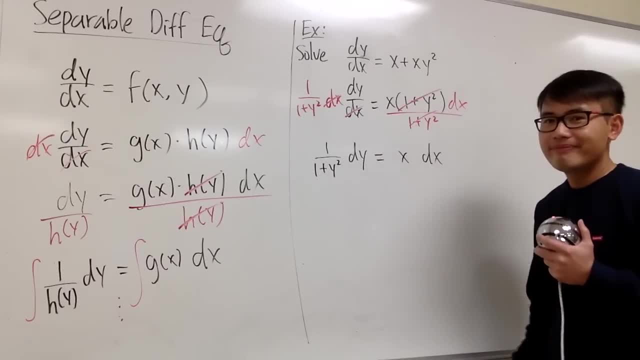 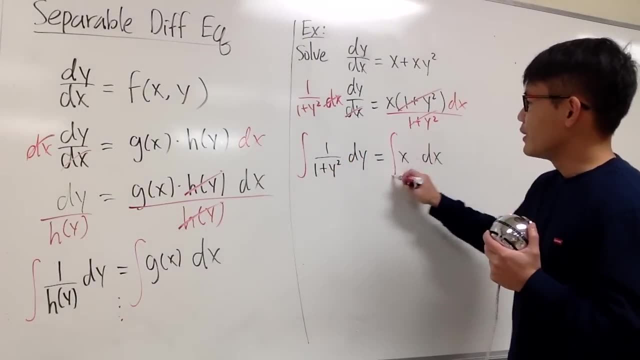 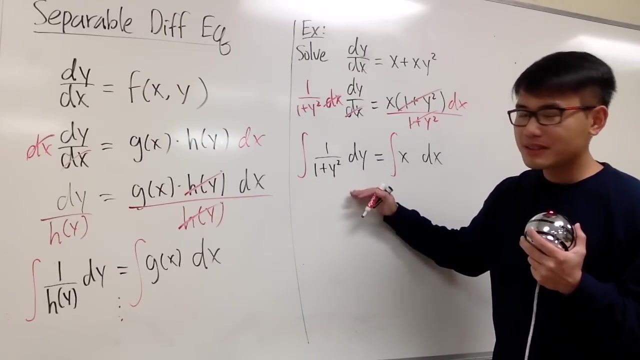 we'll have x with the dx right here, and this is what i mean by this step. okay, and now i'm just going to integrate this and integrate that and once again, i'm going to show you guys all the steps. so let's focus on this part here. first, the integral of 1 over 1 plus y, squared in the y world. 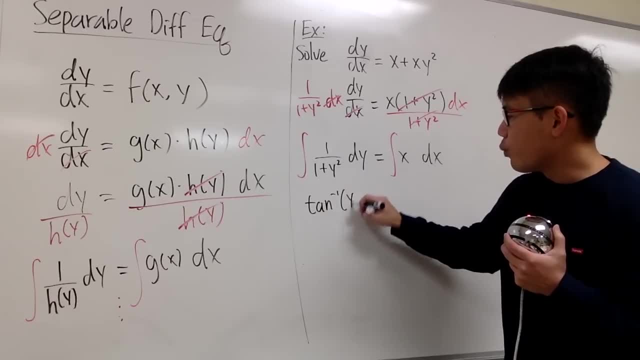 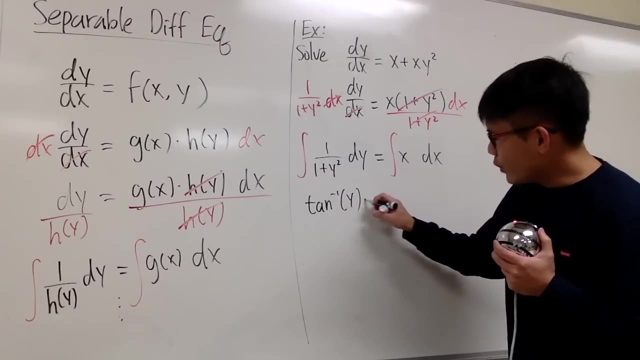 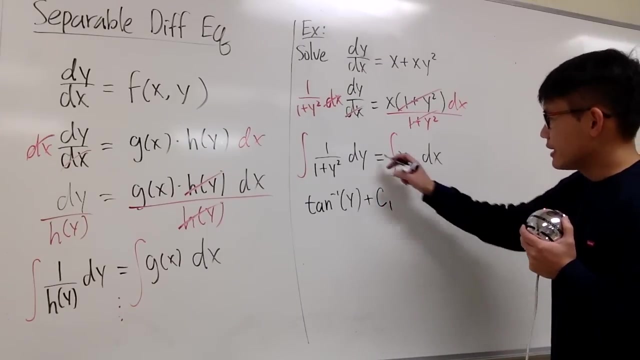 is going to be the inverse tangent of y and technically, when i integrate this, i will have to add a constant, and i will add a constant right here. but let me put this down as plus c 1.. all right, let's focus on the right hand side. this is equal. 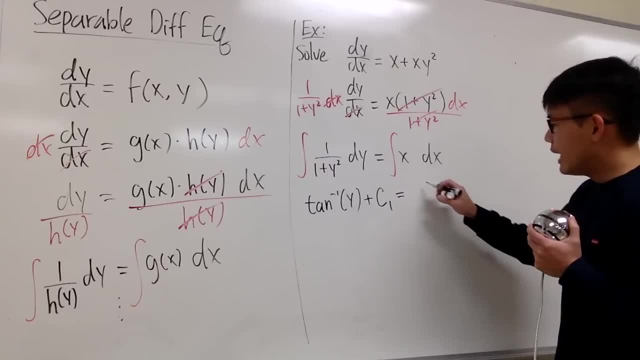 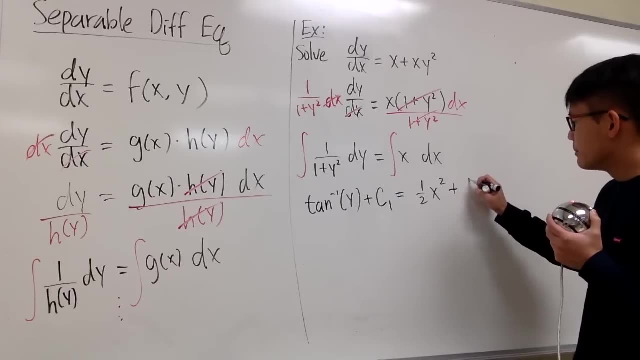 to when we integrate x in the x world, we have one half x squared, and this is the integral. we should also add a constant at the end, right? so let me add plus c, but this time it will be c 2. but, as i said, i'm just showing you guys all the steps. 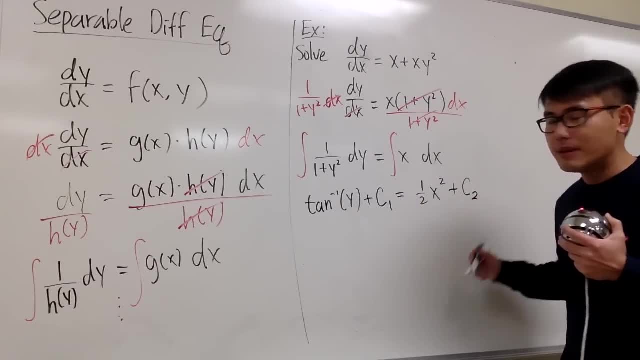 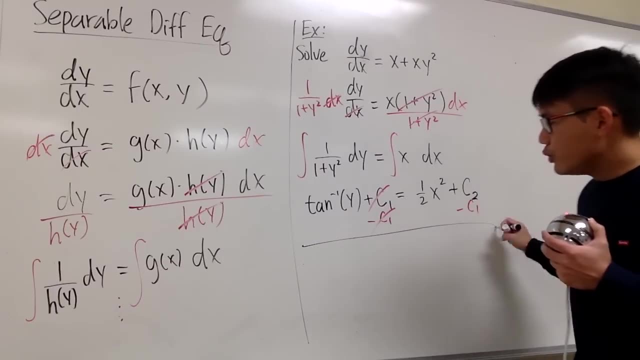 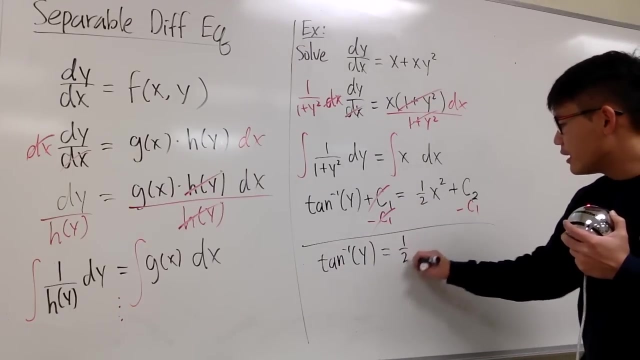 in fact, you can skip this, adding c1, adding c2 step, because what you want to do next is minus c1 on both sides so that they cancel, and you see, you will have the inverse tangent y and this is equal to one half x square. and now this is the fun part. here we 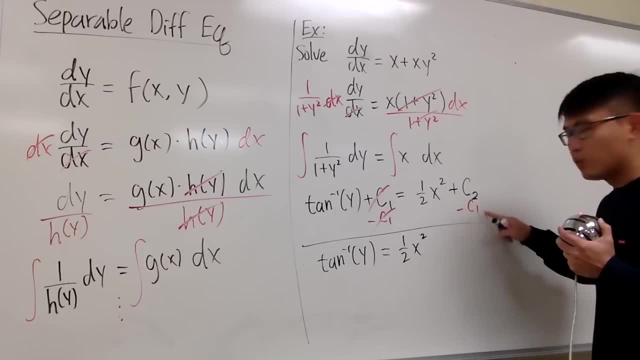 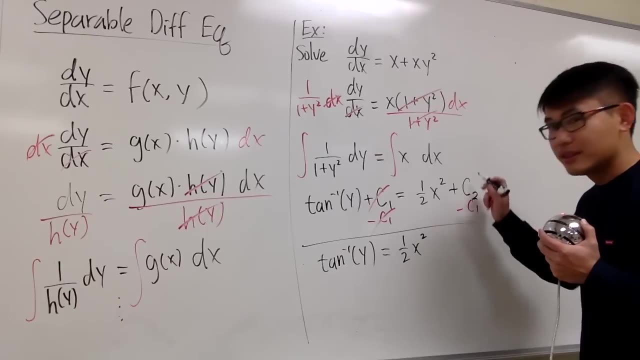 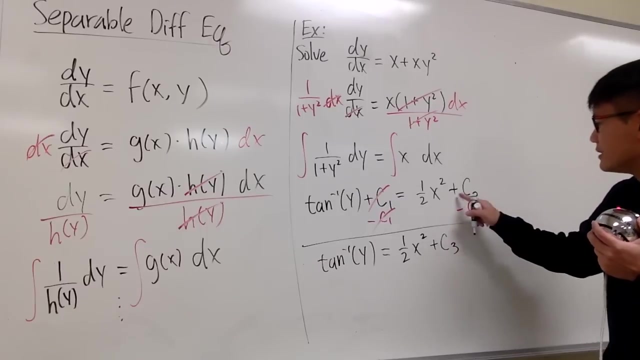 have positive c2 and then minus c1. a constant minus another constant is just another constant, so I can label this as just c3. so I can write this down as plus c3 and c3 is going to be c2 minus c1. okay, but as I said later on, you can just go. 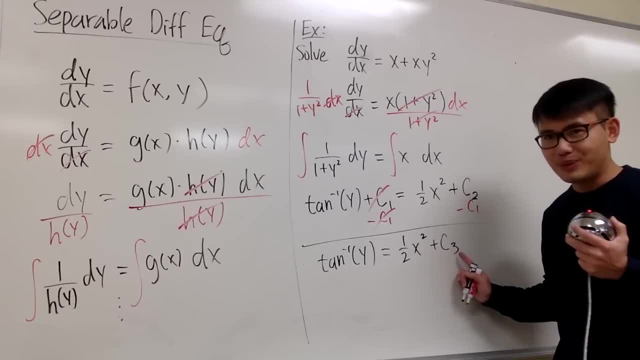 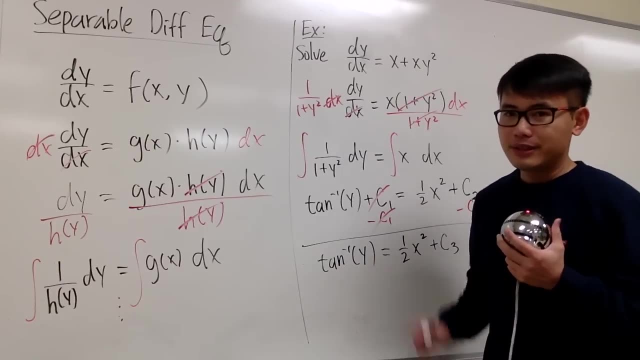 from here to here and then begin to label your constant right here as c1. but anyways, this is how I want to show you right now. well, this is not bad to isolate the y, so we will do that. let's isolate the y, so to do that, we have to. 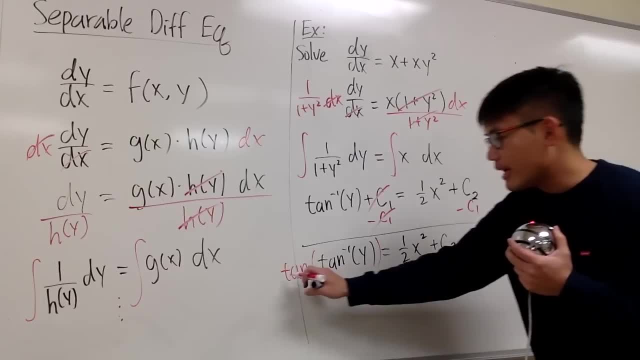 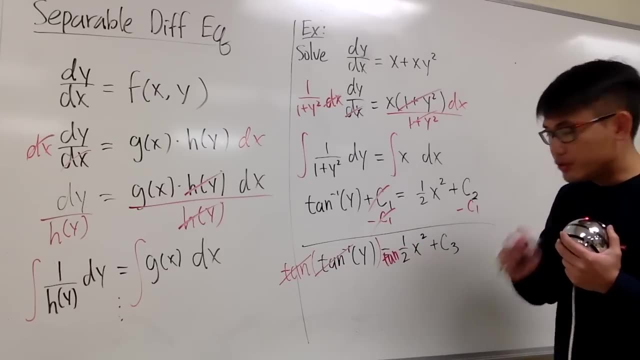 take the original tangent on both sides so that tangent and the inverse tangent will cancel. I will do that right here as well. we take the original tangent. be sure you put both the one half x square and then plus c3, both inside of the parentheses. at the end you will have y. it's equal to the original tangent of one half x. 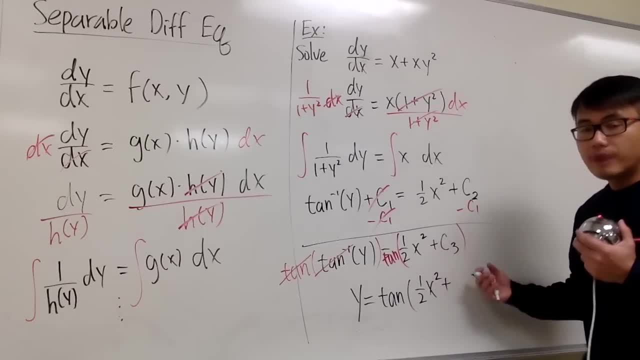 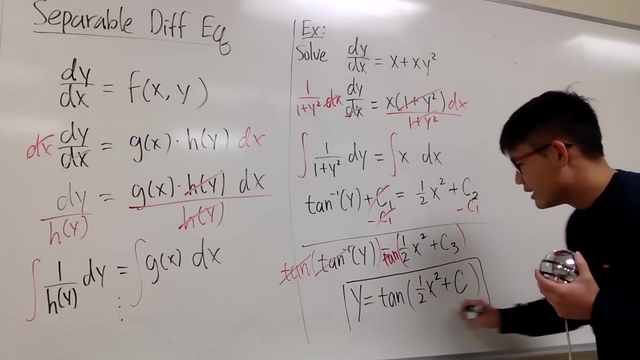 square plus c3 and we're pretty much done right. so let me just put on a c and item as a legitimate c that we want to use at the end. sometimes some books they may use a capital K right here for the final constant- up to them right, but this right here is it. this is what we mean by. 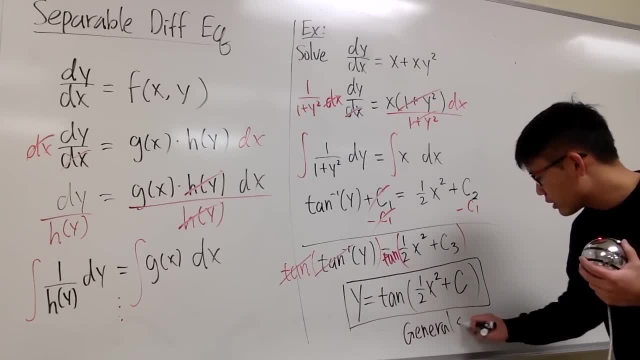 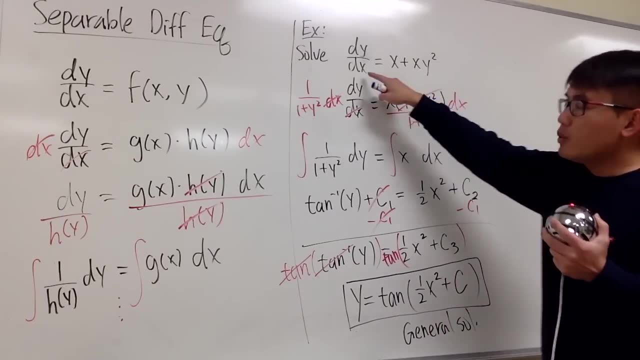 a general solution for this differential equation and this is it. however, I want to show you guys more, because suppose you're given an initial value. let's say you have this differential equation along with the initial condition. let's say y of savings, 2 goes to x and on to one half x, where there's always an initial value subs. Map the equations and fill this problem on the multiplication�. 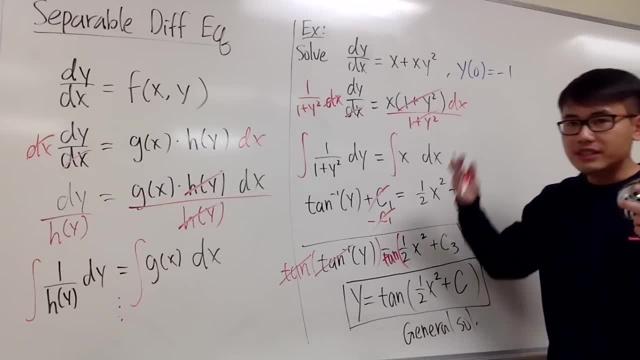 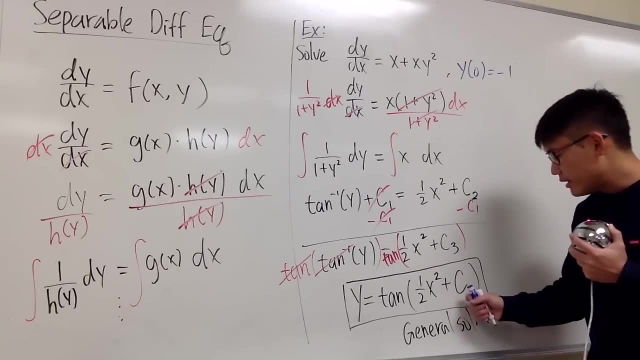 0,. this is equal to negative 1, and you want to solve this initial value problem and this is how you have to do it. Solve this. this way, we get a general solution right And our goal is to figure out what this c is. We have to use this initial condition and the way that this is written. 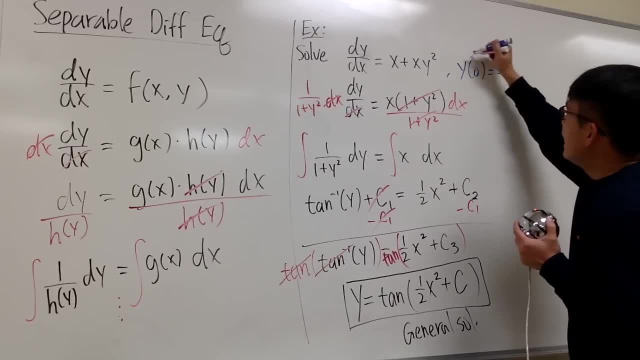 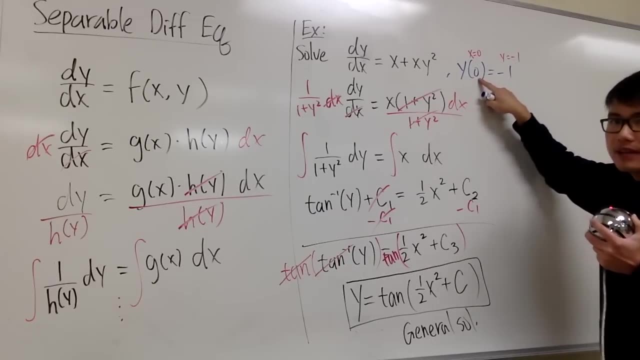 it means that when you have this 0 inside, this means x is equal to 0, and y is equal to negative 1.. y is a function of x. that's why this 0 means x is equal to 0, and the output means y is equal. 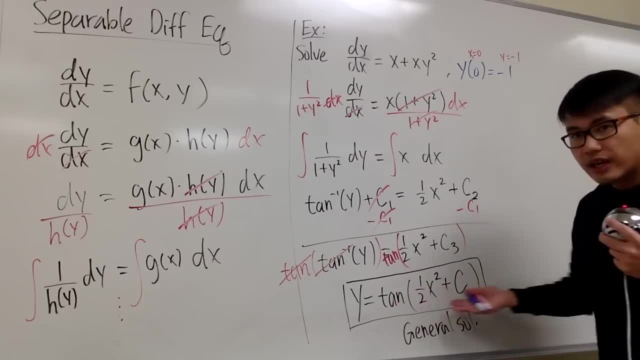 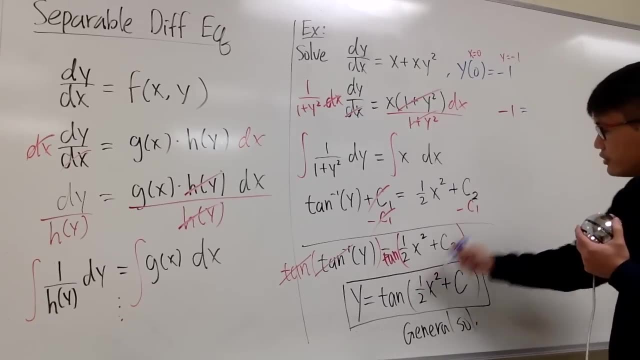 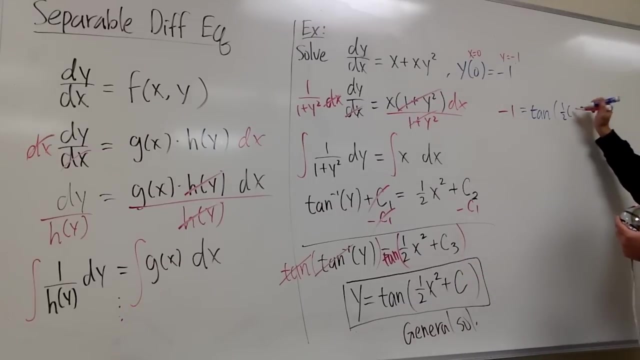 to negative 1.. Well, what do we do next? Look at the general form. Plug in negative 1 into this y here, and this is equal to tangent of 1 half and the x is equal to 0, so we're plugging the 0 right. 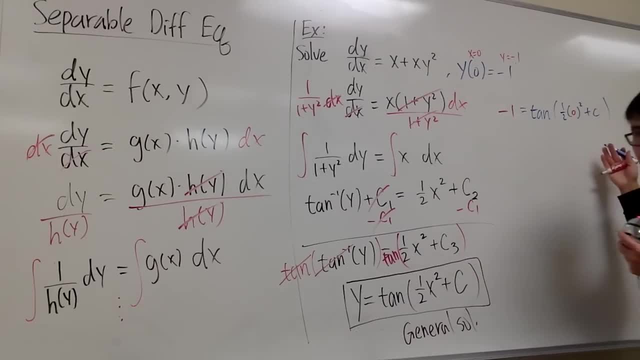 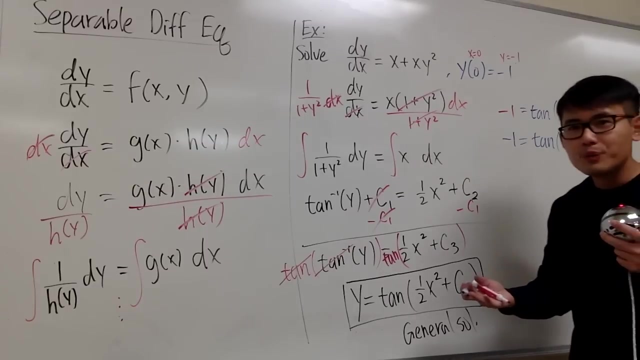 here and we'll square that and then we'll plus c, like this, right, All right. so this is going to be negative. 1 equals to tangent. this is just 0, so we just have a c inside. So negative 1 is equal to tangent c. Well, tangent of what angle will give you. 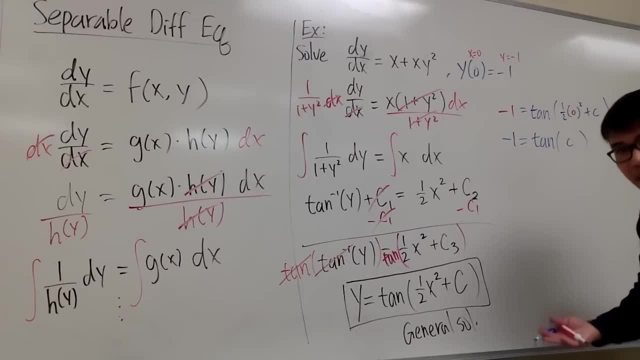 negative 1?? We know tangent of negative pi over 4 will give you negative 1, right? Therefore, c is equal to negative pi over 4.. So with this initial condition, you'll be able to find out what c is. 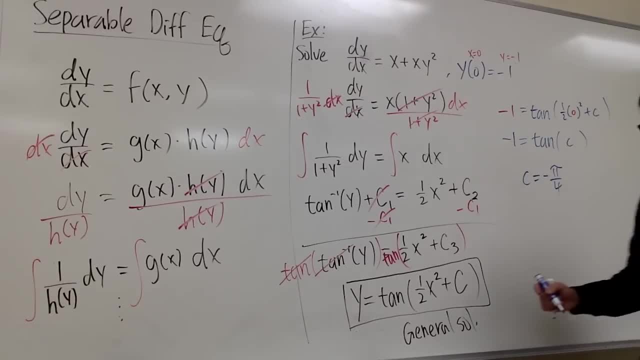 which is negative pi over 4 in this situation At the end, just plug in right here: Finally, you can say: y is equal to tangent of 1 half x squared. c is negative pi over 4, so I just have to plug in. 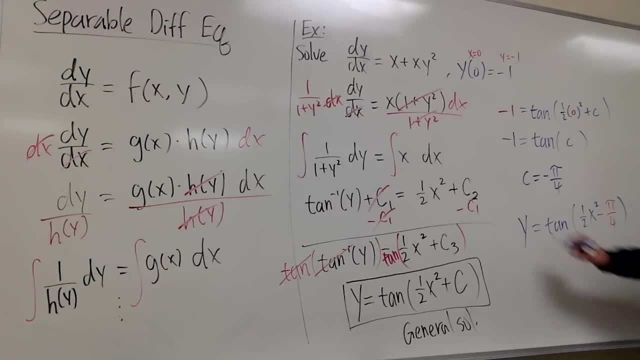 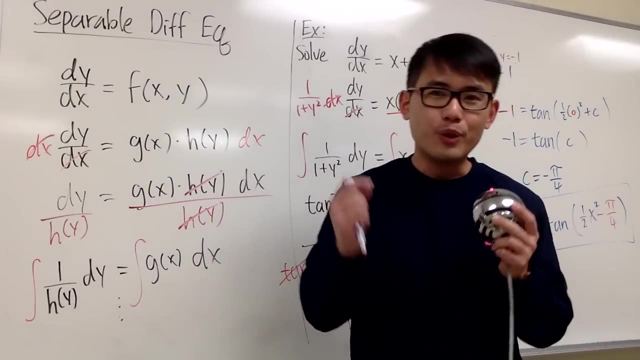 right here. So let me say minus pi over 4, like that. So this is how you solve the initial value problem and once again, I will have more videos for more examples and homework solutions for you guys.